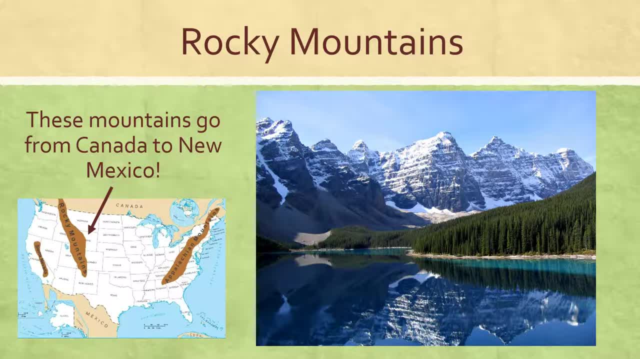 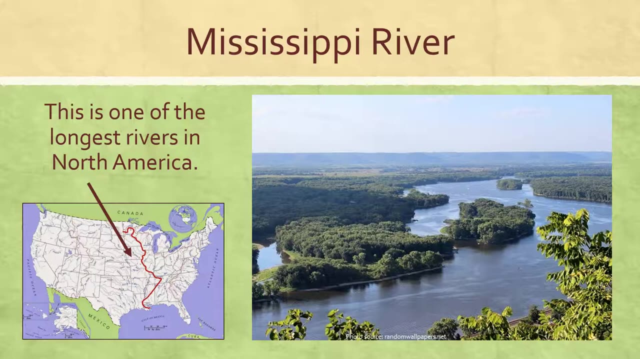 They're most famous in Colorado, where there's a lot of mountains and skiing and things like that, And these are found on the west coast or in the western part of the United States. Another geographic feature that we need to know is the Mississippi River, and this is one of the longest rivers that we've seen. 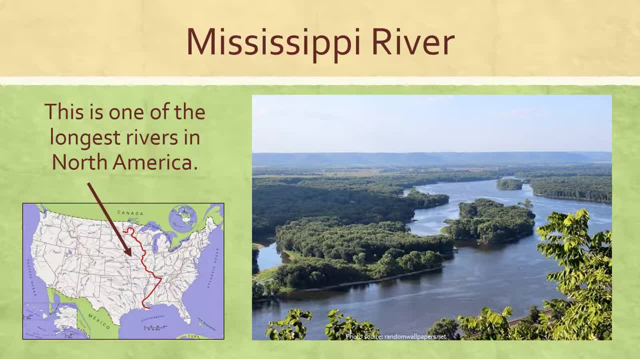 And this is one of the longest rivers that we've seen we find in North America. If you take a look at our map right here, you can see that it runs all the way from the top of the United States down through Louisiana and out into the Gulf of Mexico. 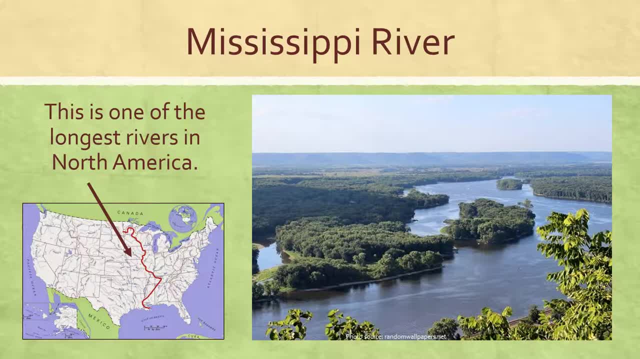 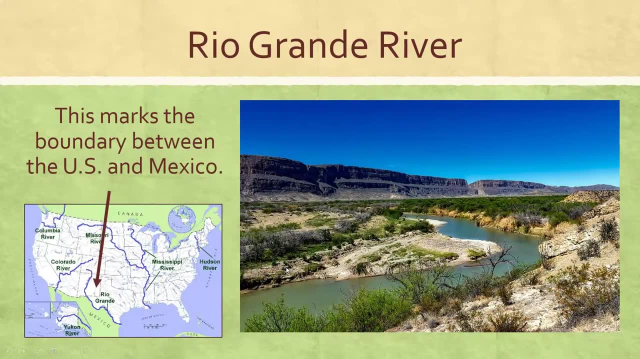 It is a giant river. In fact, it is the third longest river in the world. That's the Mississippi River. The other river that you need to know is called the Rio Grande and it flows through the Rocky Mountains from Colorado down through New Mexico, and then it actually helps to form the 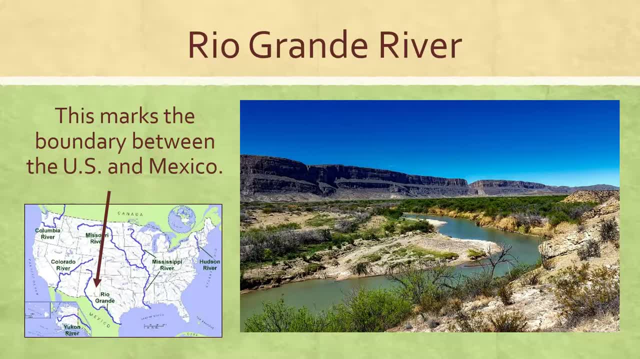 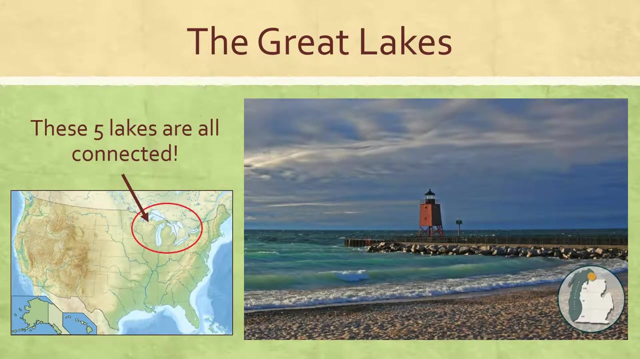 border between Texas and the country of Mexico. It flows right there along the southwestern part of Texas to help give it a border and to separate Texas from the Mississippi River. And then in the northern part of our country, in the northern part of North America, we have these. 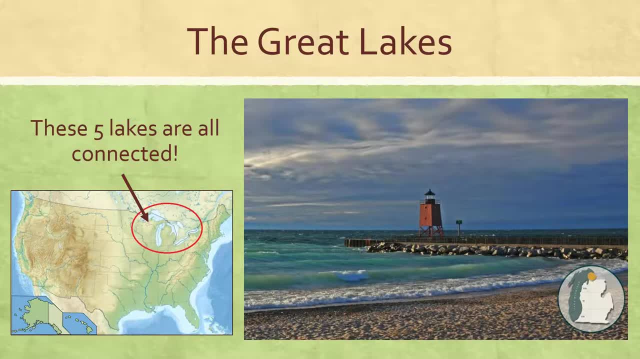 five lakes that are all connected, known as the Great Lakes, And these lakes are quite large, Hence the name the Great Lakes. We have Lake Ontario, Lake Superior, Lake Huron, Lake Michigan and the Great Lakes. There is one more that, for some reason, I cannot remember. Oh dear, that's going to bother me. 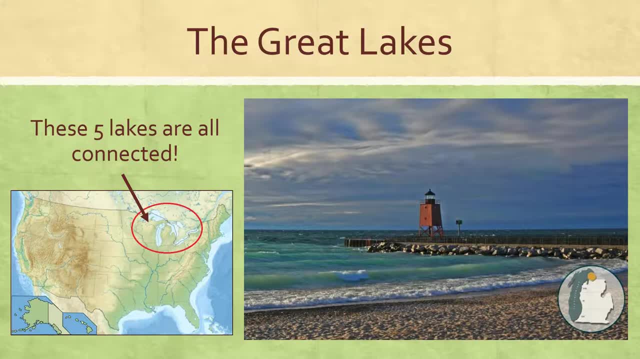 So Lake Ontario, Lake Michigan, Lake Huron, Lake Superior and Lake Erie. There we go. Let me say those again: Lake Erie, Lake Superior, Lake Huron, Lake Michigan and Lake Ontario. Those are known as the Great Lakes and they are located in the northern part of. 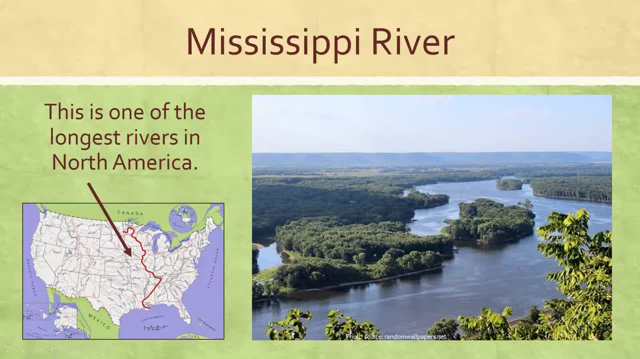 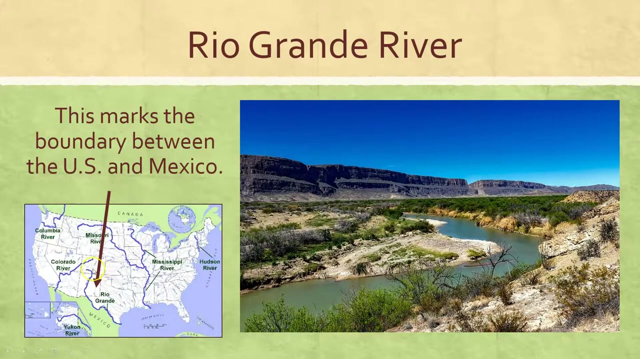 the way from the top of the United States down through Louisiana and out into the Gulf of Mexico. It is a giant river. In fact, it is the third longest river in the world. That's, the Mississippi River. The other river that you need to know is called the Rio Grande and it flows through the 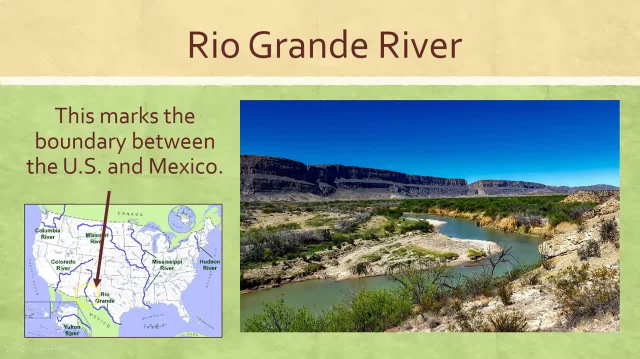 Rocky Mountains, from Colorado down through New Mexico and then it actually helps to form the border between Texas and the country of Mexico. It flows right there along the southwestern part of Texas to help give it a border and to separate Texas from the Mississippi River. 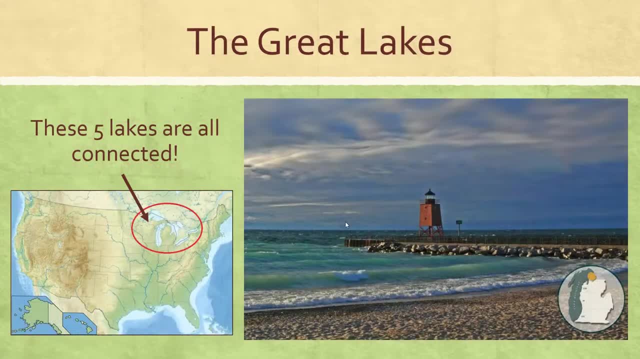 And then in the northern part of our country, in the northern part of North America, we have these five lakes that are all connected, known as the Great Lakes, And these lakes are quite large, Hence the name, the Great Lakes. We have Lake Ontario, Lake Superior, Lake Huron, Lake Michigan. 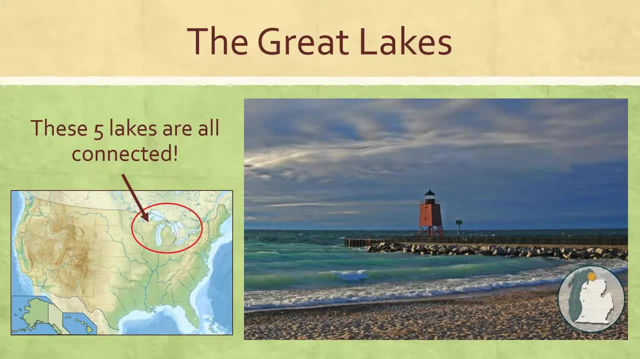 and the Great Lakes. There is one more that for some reason I cannot remember. Oh dear, that's going to bother me. So Lake Ontario, Lake Michigan, Lake Huron, Lake Superior and Lake Erie. There we go, Let me say those again: Lake Erie, Lake Superior, Lake Huron, Lake Michigan and Lake Ontario. 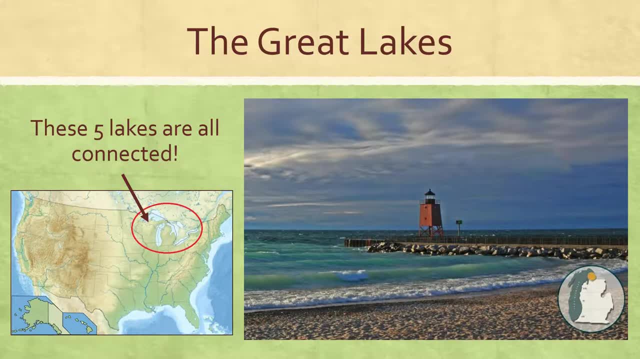 Those are known as the Great Lakes and they are located in the northern part of North America, the northern part of the United States. So again, we have five geographic features. We have the Appalachian Mountains, If you look here on the map that I'm pointing to. 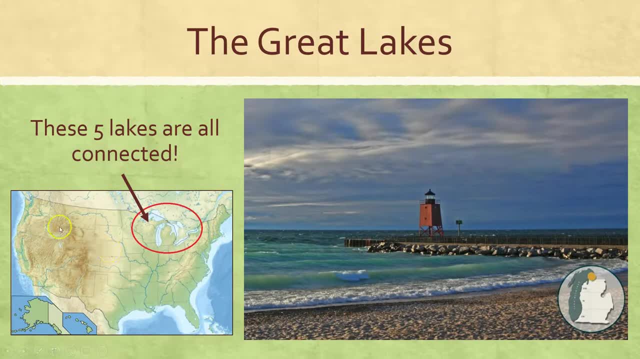 they run down the east coast of the United States. Over in the western part, over through here, we have the Rocky Mountains. They go from Canada down to New Mexico. Then we have the Mississippi River, which is the third longest river in the world. It's also one of.